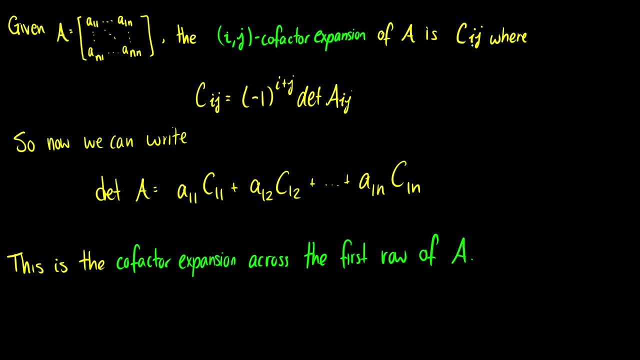 with subscripts ij, where cij is equal to negative, 1 to the i plus j times the determinant of capital, Aij. So how is this different than just Aij, or, in fact, the original expression? Well, now we're able to write the determinant of A as A11, c11 plus A12, c12 plus, all the way up to. 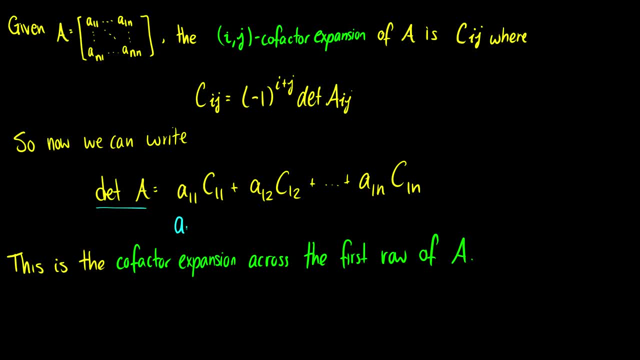 A1n, c1n. So no longer do we have to write the determinant of A11 and then subtract and add and subtract every other term. So let's go ahead and do that. So let's go ahead and do that. So the point here is that using the c11, we can just plug our row and column into the formula to: 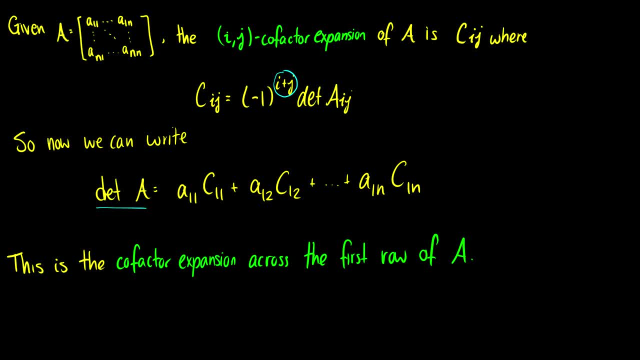 figure out if we have to add or subtract. Also, now we don't have to do it exactly across the first row. So this example here is the cofactor expansion across the first row, And it's across the first row because our first entries are all going to be in the first row. So it goes from 1,. 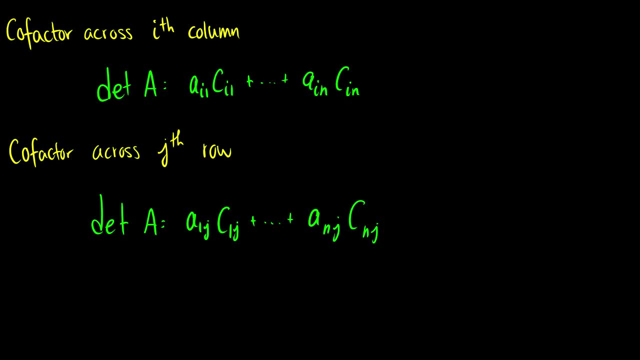 1 all the way up to 1n. The nice thing is that we can do this again around the ith column or across the jth row. We can do this forever. So why can we do this? Well, before, if we did this, we'd have to count. We'd have to say, OK, this one's plus this one's. 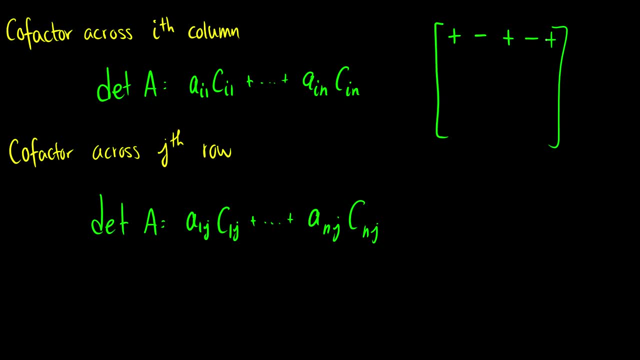 minus this one's plus this one's minus this one's plus, so on and so forth. However, with our formula, so remember, we have negative 1 to the i plus j. Well, now we can say: OK, what is the A46? 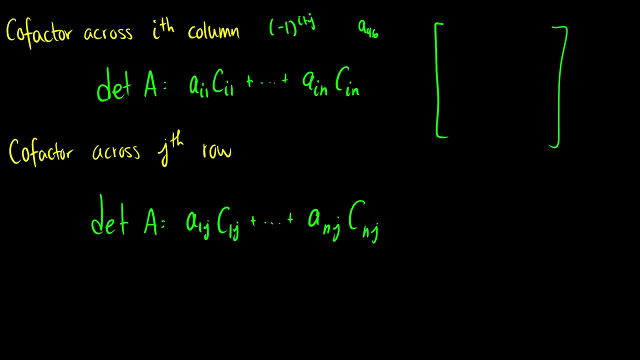 entry going to be. Is it going to be positive, Is it going to be negative? Is it going to be positive? Well, it's going to be negative: 1 to the 4 plus 6, which is negative 1 to the 10.. So this entry. 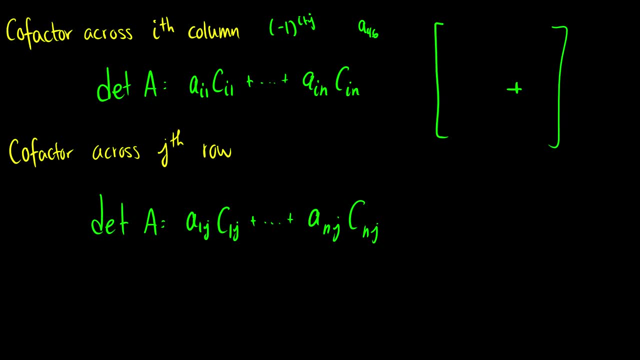 here A46, is going to be positive, So that's what we can do with this. So now we can do cofactor expansion and find the determinant along the ith row, So we hold the ith row constant here. or across the jth row, So we'll hold the jth row constant. So now we can do cofactor expansion. 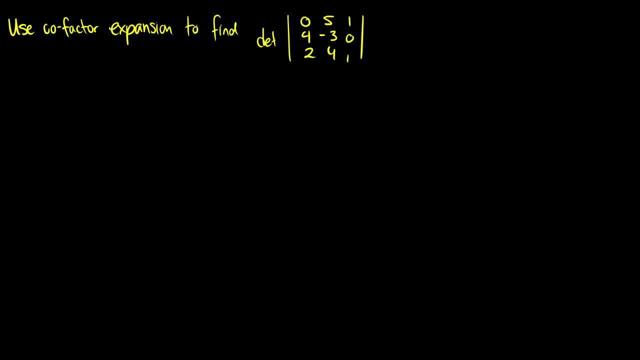 wherever we want. So when is this useful? Well, let's use cofactor expansion to find the determinant of this matrix. So what's good about this is now we use zeros to our advantage. So I see a 0 in the A11 column. 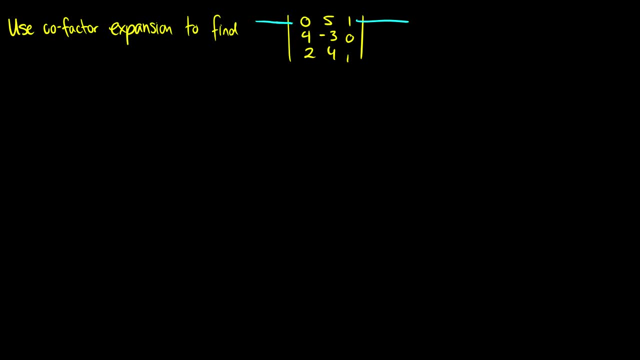 So what I'm going to do is I'm going to do cofactor expansion across the first row. So our 0, 5, 1, 4, negative 3, 0, 2, 4, 1.. 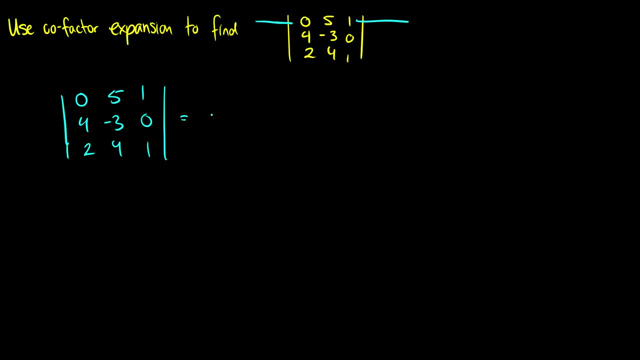 OK, so let's write this out formally: This is going to be A11, C11, plus A12, C12, plus A1C, C13.. OK, so what is A11?? It's 0.. So C11 doesn't matter. A12 is going to be 5.. OK. 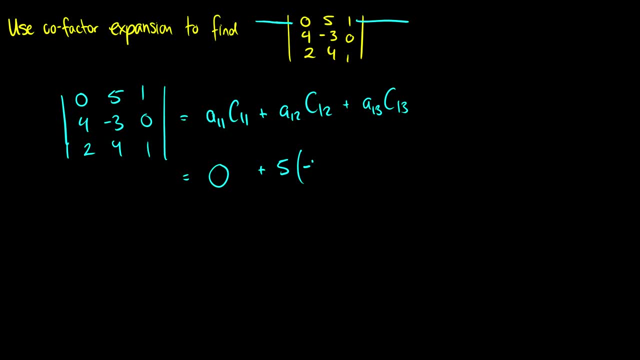 so what's C12?? Well, remember, it's negative 1 to the power of i plus j. So that's going to be negative 1 to the 1 plus 2.. And then we have to multiply that by the determinant of the submatrix A12.. 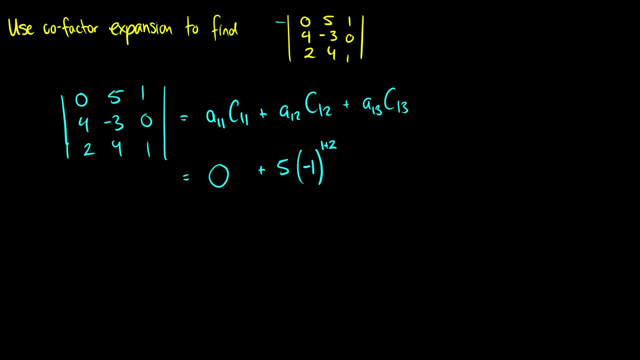 So in this case, A12 means we take out the first column, or the first row, and the second column, So we're going to be left with 4, 0,, 2,, 1.. And then, finally, we're going to add A13.. A13 is just 1.. C13 is going to be negative 1 to the power of 1 plus 3.. 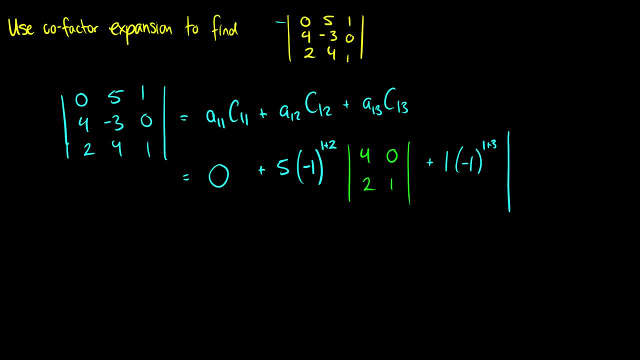 And then we'll multiply this by the submatrix A13.. So that's not the first row, not the third column. So we're left with 4, negative 3, 2, and 4.. OK, so this is going to be 0 for the first term, 5 times negative 1 to the power of 3.. 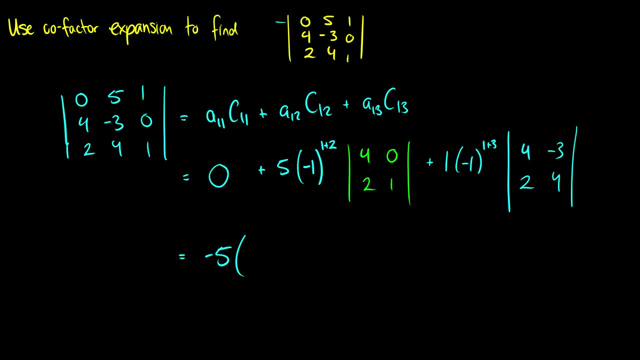 It's going to be negative 5.. The determinant of 4, 0, 2, 1 is going to be 4 times 1 minus 2 times 0. Then we're going to add, And then we're going to add. 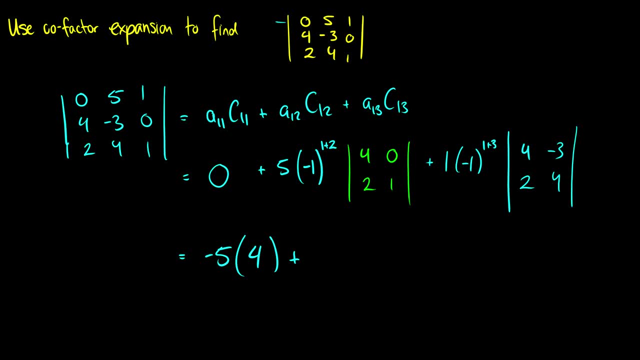 Well, negative 1 to the power of 4 is 1.. So we're just going to end up adding the determinant of 4, negative 3, 2, 4.. So it's going to be 4 times 4 is 16 minus 2 times 3.. 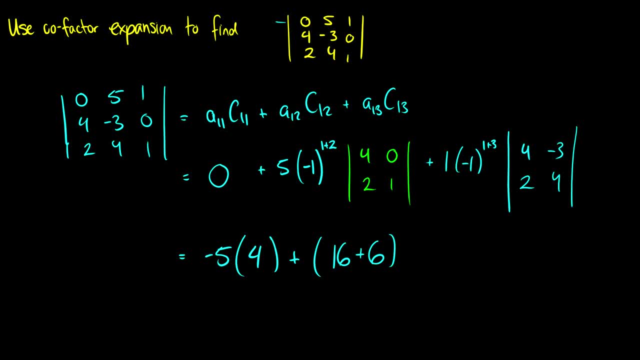 That's negative 6.. So we're going to subtract negative 6, which is the same as adding 6. So here we get negative 20 plus 22.. So our determinant is going to be equal to negative 2.. So another note here. 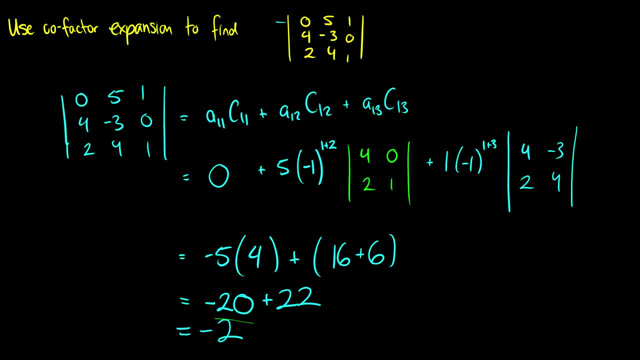 I said before that determinants can be really big. They can also be negative, So that's OK, But because, again, this is not 0, we know that this matrix is going to be invertible. So, again, another point that I made last time is, if the determinant is not equal to 0, then 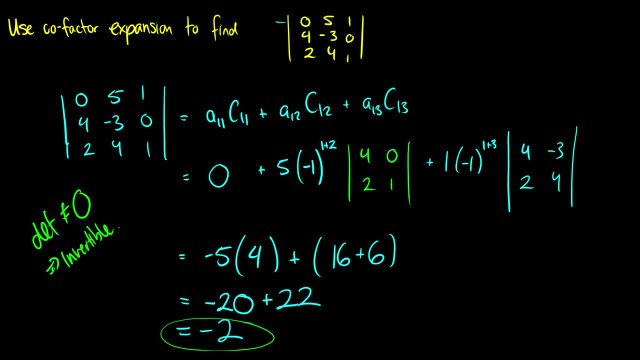 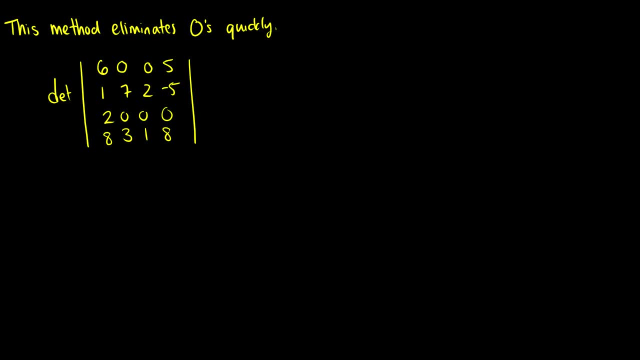 the matrix is invertible. So these are just side points I'll bring up to remind you every once in a while. OK, So that's nice. OK, So this is going to be 1, 0, but we can do so much better. 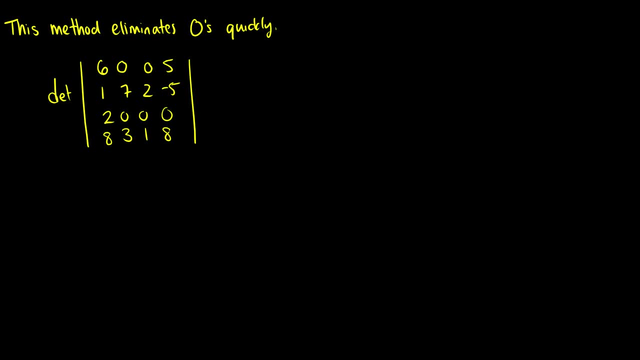 So look at this matrix here: 6, 0,, 0, 5.. This is really good. This is a great line. It has two 0s in it And we have 1,, 7,, 2, negative 5.. 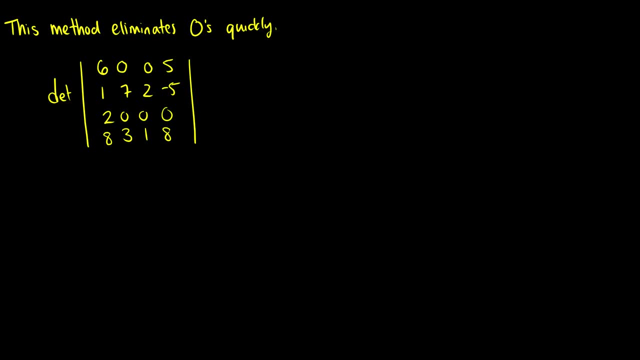 But here we have 2, 0, 0, 0.. Let's do cofactor expansion across this third row here. So, OK, This is going to be c, or I guess we'll call this a31 times c31.. 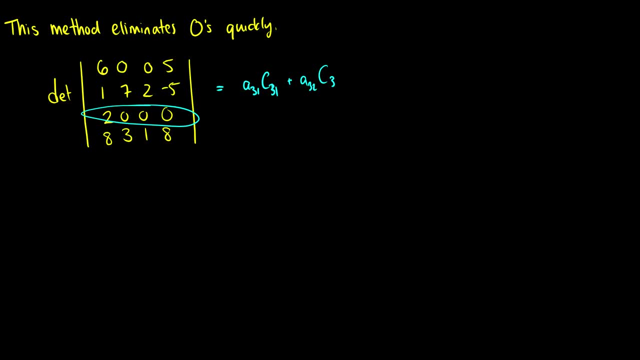 Plus a32 times c32, plus a33 times c33, plus a34 times c34.. So that's cofactor expansion across the third row, OK, c31.. This is going to be 2.. Then we have to multiply this by the determinant of the submatrix of a31.. 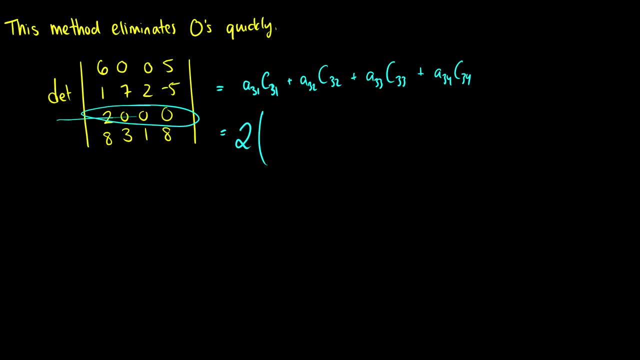 So in this case, here we get rid of the third row And the first column. So now we're left with the determinant of 0, 0,, 5,, 7, 2, negative 5, and 3, 1, 8.. 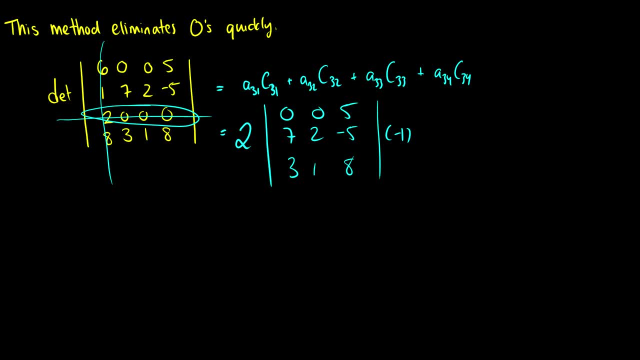 And then, of course, I also have to take negative 1 to the power of i plus j, which will be 3 plus 1.. OK, So that's a31, c31.. Now we need to do the next one. 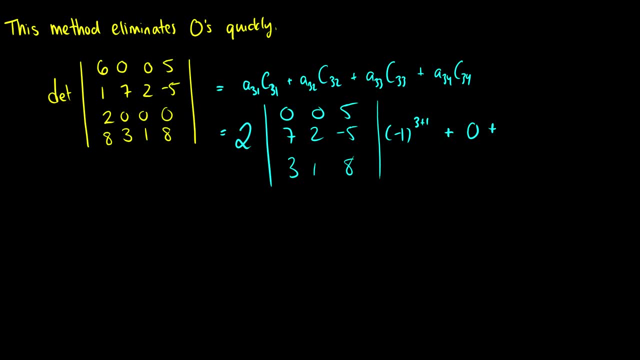 OK, 0.. So that's done. a33 is 0.. a34 is 0.. So those will all be 0.. And look Now: with one operation and one calculation, we have reduced this to 2 times the determinant. 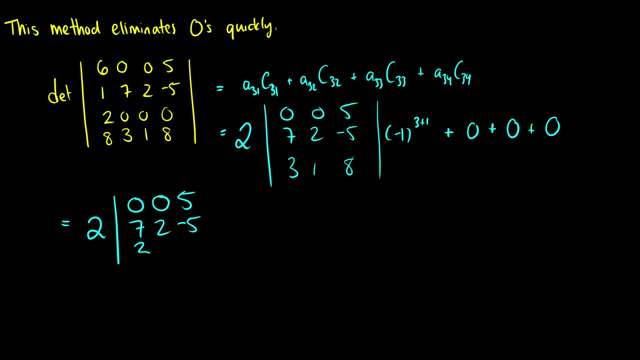 of 0, 0,, 5,, 7,, 2, negative 5, 3,, 1, 8.. But it gets even better Because now we have another row we can do this with. We have 0, 0, 5.. 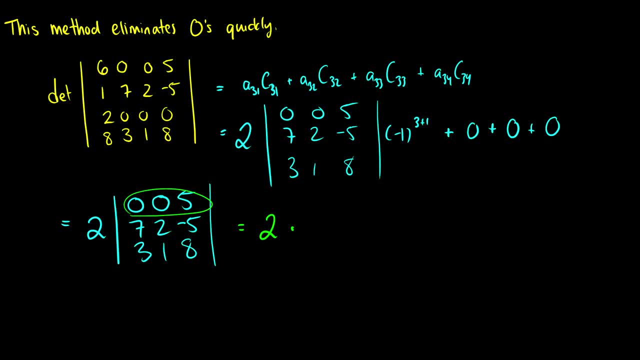 So this is going to be 2 times a11, a11, or, I guess, a11, c11, plus a12, c12, plus a13, c13.. But at this point, well, 2, a11 is 0, a12 is 0. 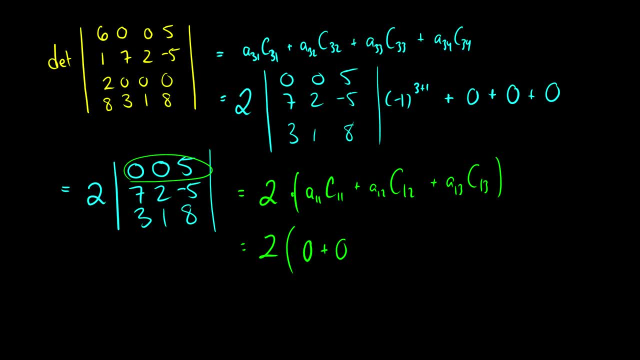 So all we have to do is a1, c3, sorry, a13, c13.. That's going to be 5 times 0.. OK, 0, 0, 5 times. well, negative 1 to the i plus j, so it's 1 plus 3.. 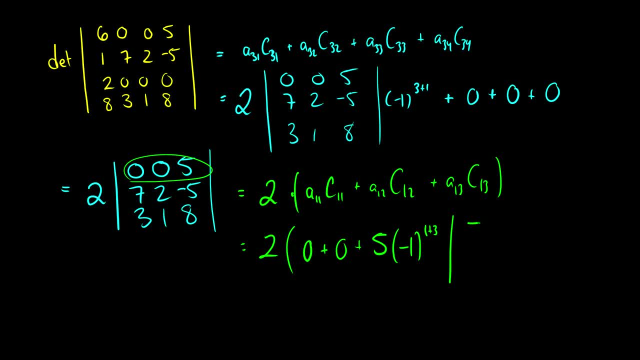 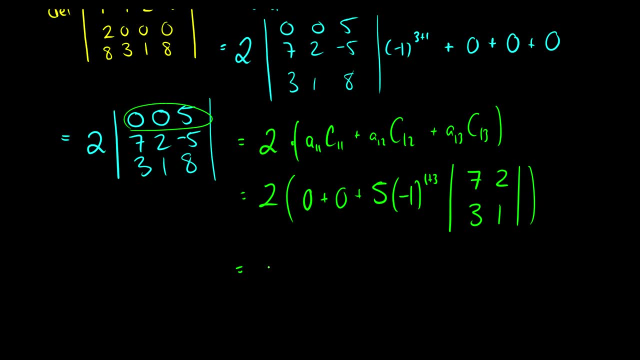 And then the determinant taking out the first row and the third column. So we're going to be left with 7, 2,, 3, 1.. All right, So now, at this point, this is going to be 2 times 0, 0 plus 5 times negative 1 to the. 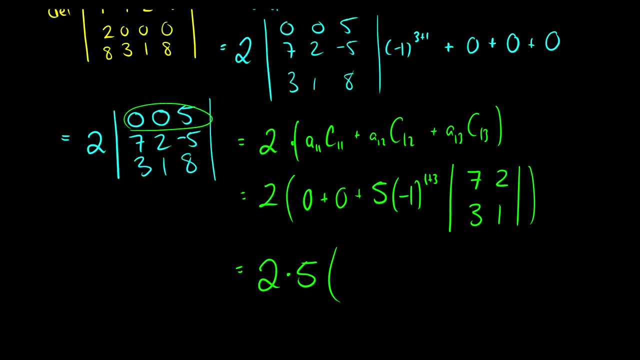 4. That's 5 times the determinant of 7, 2, 3, 1,, which is going to be 7 times 1.. Minus 3 times 2,, that's 6.. So our determinant is going to be 10.. 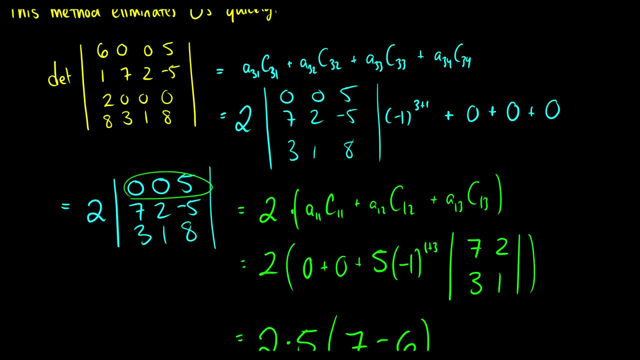 So with cofactor expansion we made this a lot easier, Because before we would have had to go across the top first, So we would have had to do 6 times this submatrix and then minus plus minus 5 times this submatrix. 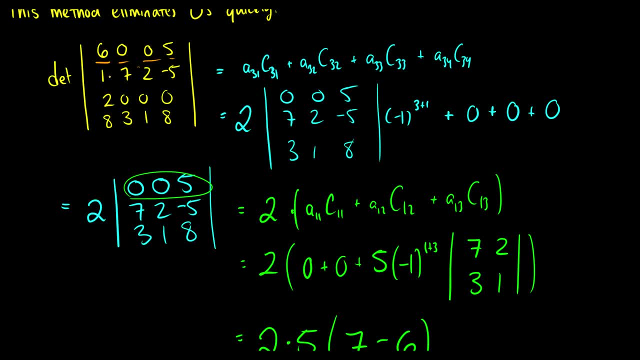 And then we would have had to do the determinant of two of these submatrices And we would have had to move across the top row here. So we never would have been able to simplify our work, And doing this by hand would have taken a lot longer. 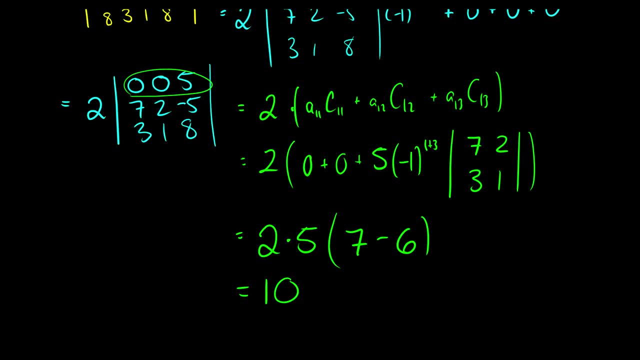 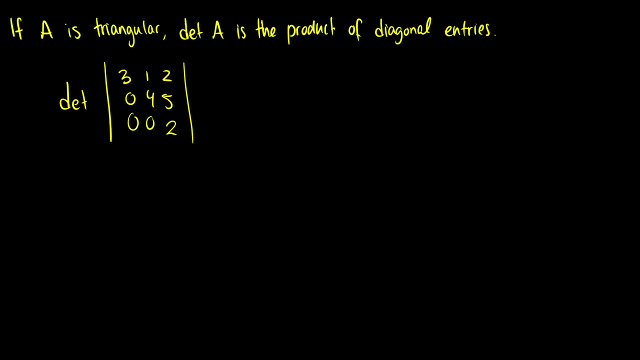 So on exams, cofactor expansion is your best friend. Pick the easiest lines and do it OK. So one last theorem: If A is triangular, then the determinant of A is the product of diagonal lines or diagonal entries. So if I take a look at the determinant of this, this is just going to be equal to 3. 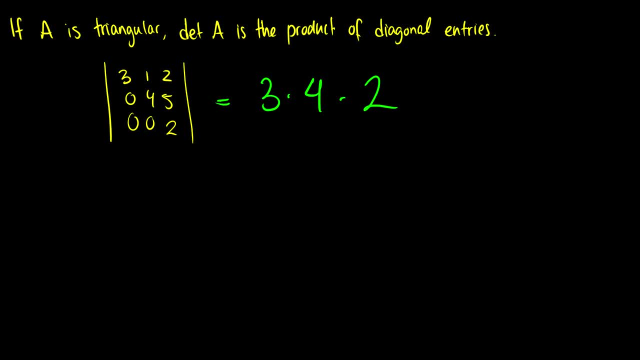 times 4 times 2, because these are the diagonal entries. Now, why is this the case? Well, we could do this generally. So if you want to make a proof of a general example, you can, But I'm going to do this with this example. 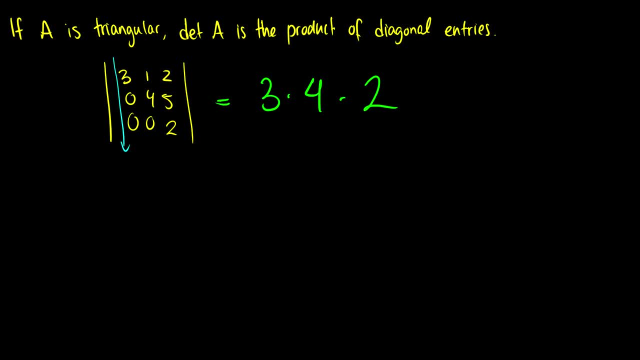 So first we can do cofactor expansion down the first column. So this is going to be A117.. OK, C11 plus A21, C21 plus A31, C31.. So these A21s and A31s, these are going to be equal to 0. 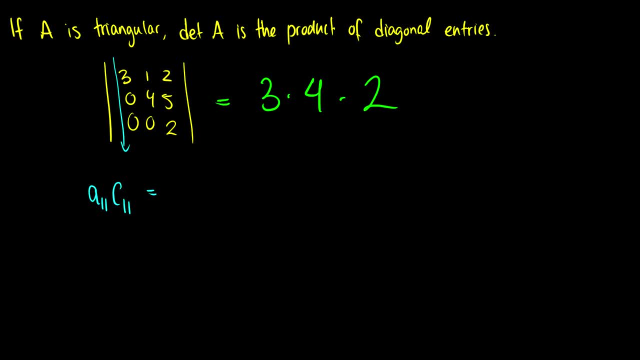 So we really just have to look at A11, C11.. And this is just going to be 3 times negative: 1 to the 1 plus 1 times the determinant of 4, 5.. 0, 2.. So this is just equal to 3 times the determinant of 4, 5, 0, 2.. 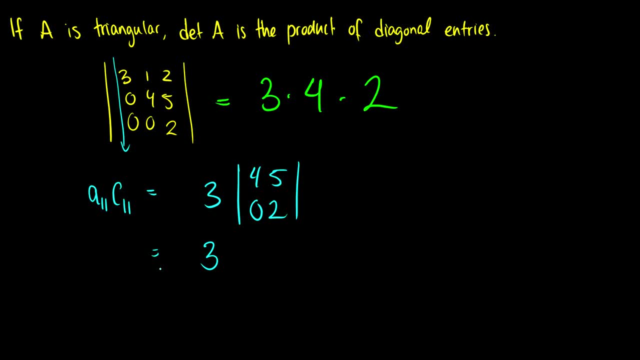 And again, what's the determinant of 4, 5,, 0, 2?? Well, this is just going to be 4 times 2 minus 5 times 0. So this is equal to 3 times 4 times 2.. 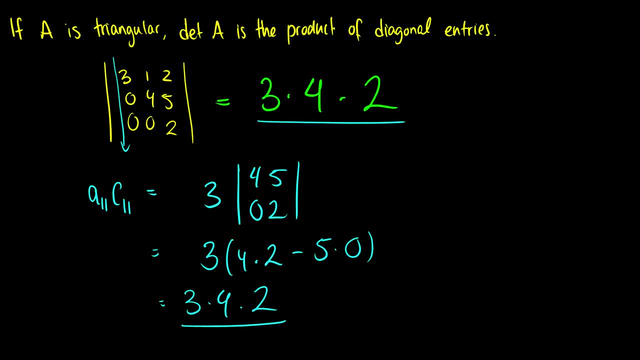 So this was not a full proof of this. This was just an example that shows the proof to be true. But if you wanted to do this, you would start with induction on something like A11,, A12,, A21, A22.. 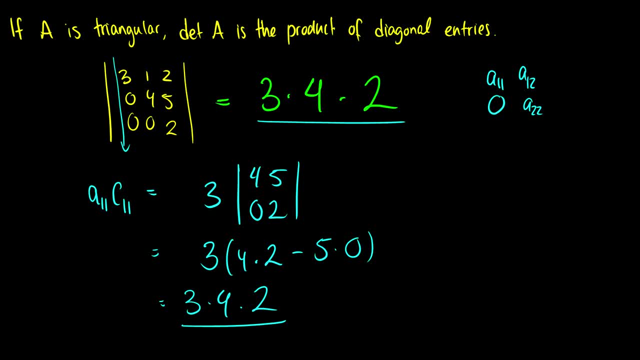 So this would be 0, of course. So you can do induction with this, So you'd show the base case, And then what you do is you'd assume for a smaller matrix, that's say A22, all the way down to ANN, is true?